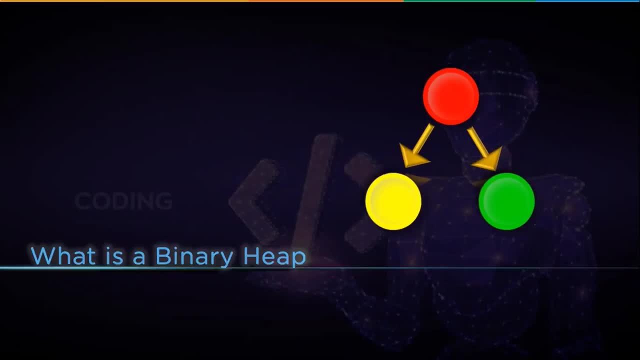 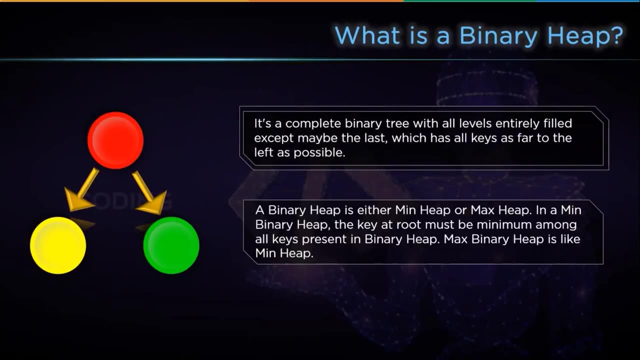 Simply Learn. So, without any further ado, let's get started with. what is a binary heap? It's a complete binary tree with all levels completely filled, except the last level Where all leaves are to the left. as far as possible, A binary heap can be either min heap or max heap. In a min binary heap, the elements at root- 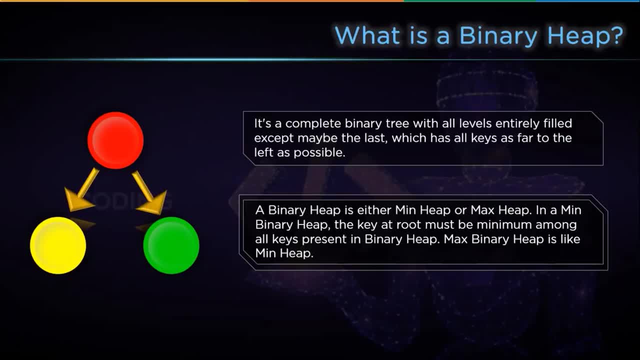 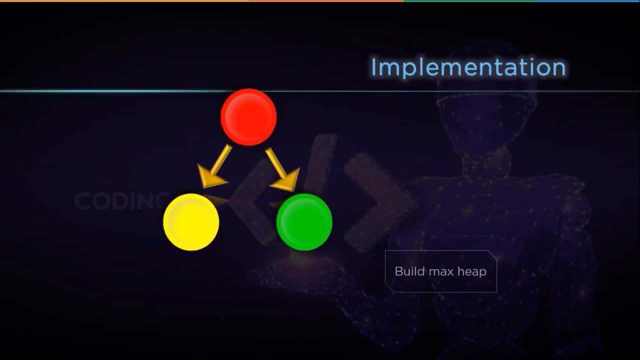 must be minimum among all elements present in the binary heap. Max binary heap is like min heap, where root must be maximum among all elements. Now let's discuss implementation of heap sort. First, we will start with creating a max heap of elements present. Next up, we will remove the elements at the root and put it at the end of the array and put the smallest element at the root. After that, we will reduce the height by 1.. Finally, we will heapify the root element again and repeat the process from step 2.. Now let's try. 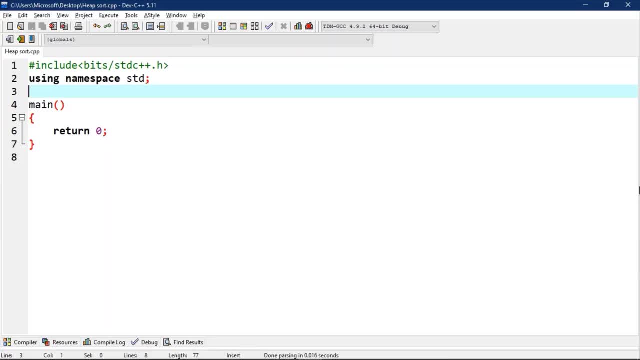 implementing this algorithm in the code editor. We will start by creating a function to heapify a subtree rooted with node i, which is an index in array arr and n is the size of the heap. So void: heapify: int, arr, comma int, n, comma int. 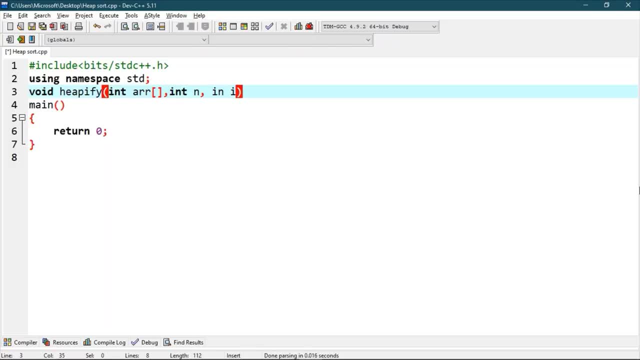 int i. Now we will initialize largest as root. so int largest i. Now we will define the left and the right subtree. So int l is equal to i to 2 into I plus 1 and int r is equals to 2 multiply with I plus 2.. Now if the left 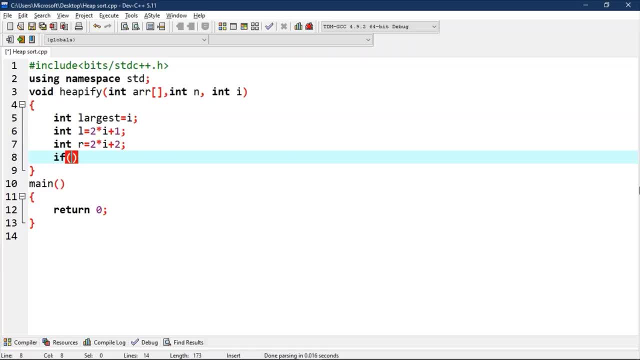 child is larger than root than if l is less than n, and arr at l is greater than arr at largest. Now, if the left child is larger than root than if l is less than n and arr at l is greater than r, so the largest will be equals to l. 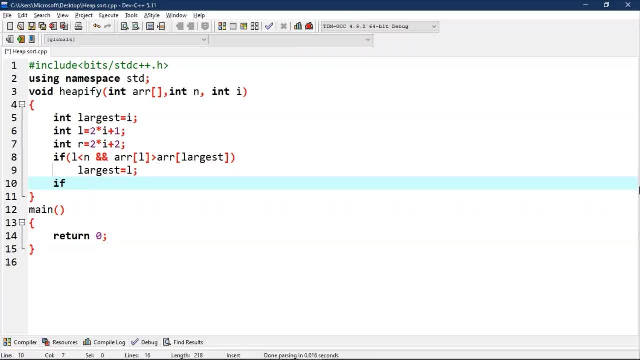 Now if right child is larger than the largest so far. so if r is less than n and arr at r is greater than arr at largest, So largest is equals to r. Now if largest is not roo, So if largest is not equals to I. 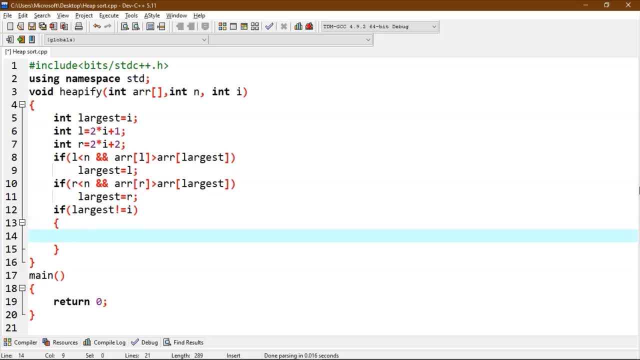 So we will swap arr at i with arr at largest and then we will recursively call epify for the affected subtree. here are comma n, comma largest. Now we will write the main function to do heap sort. so void. Now we will write the main function to do heap sort. 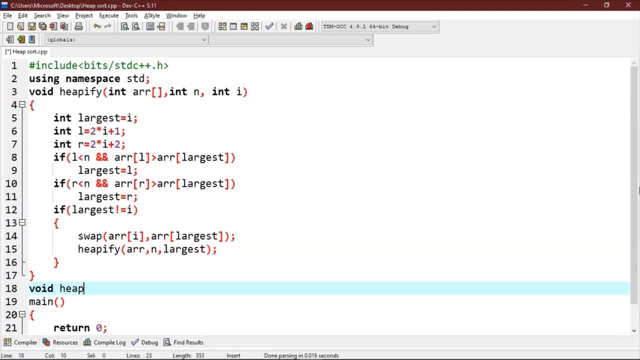 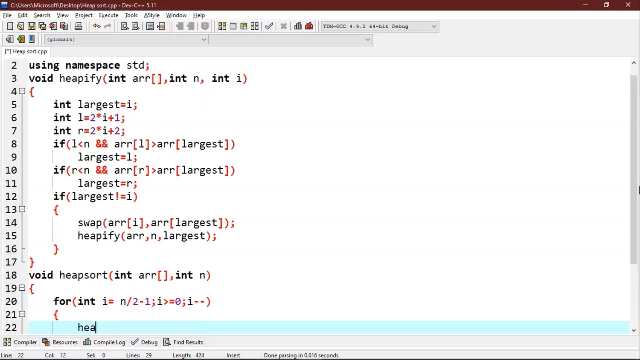 int. arr bracket, comma int n. Now we will start by building heap. so for int i is equals to int By n, By n, By n By 2, By 1, Where i is greater, then equals to zero at i. We will call mä For arr end end. 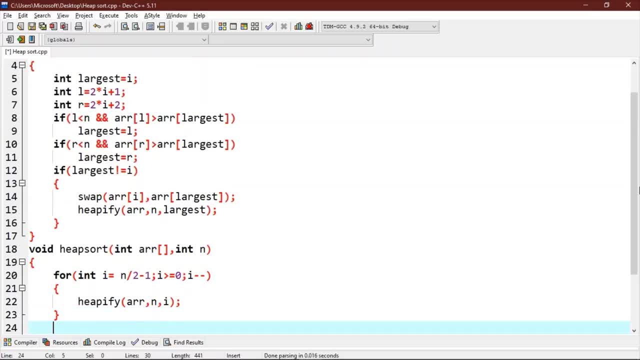 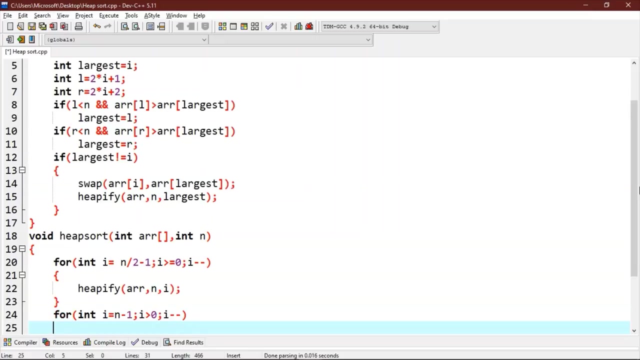 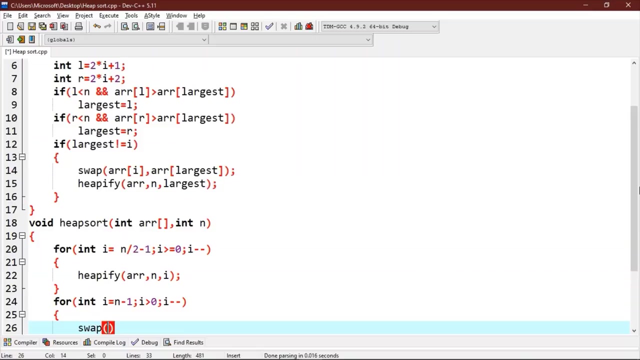 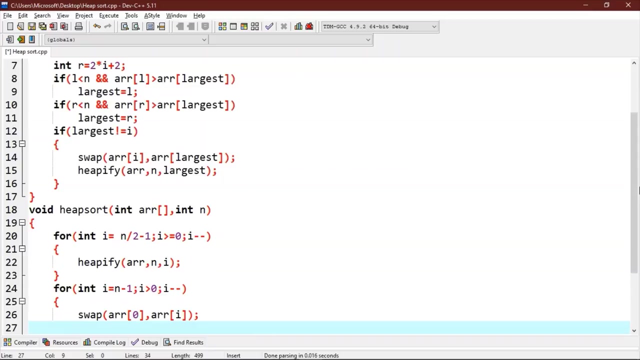 By 2. Now we will one by one extract an element from the heap. So for int, i is equals to n-1, where i is greater than 0 at i-minus. Now we will move current root to n, so swap arr at 0 to arr at i and we will call max. 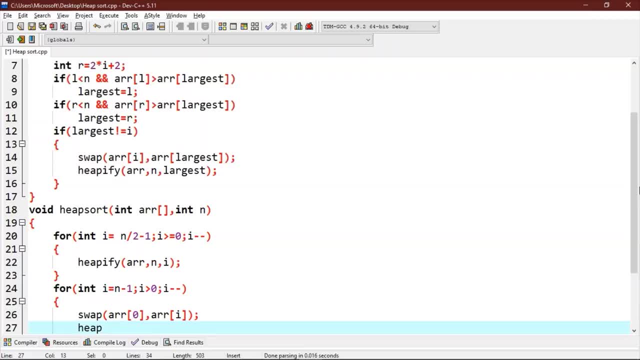 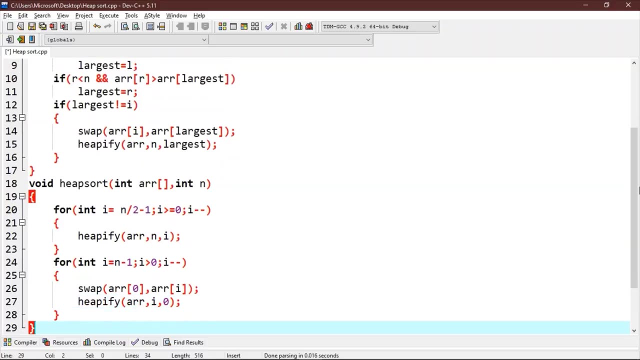 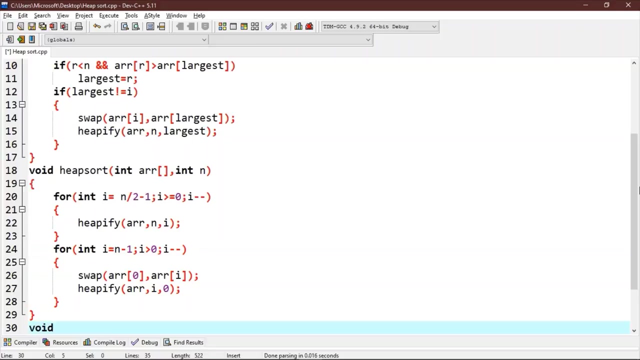 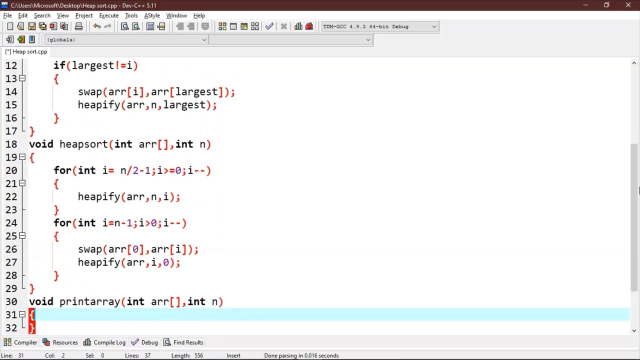 heapify on the reduced heap, So heapify arr comma i, comma 0. Now we will write a function to print this array. So void int array, int arr comma, int n. So for int i is equals to 0 at i-minus. 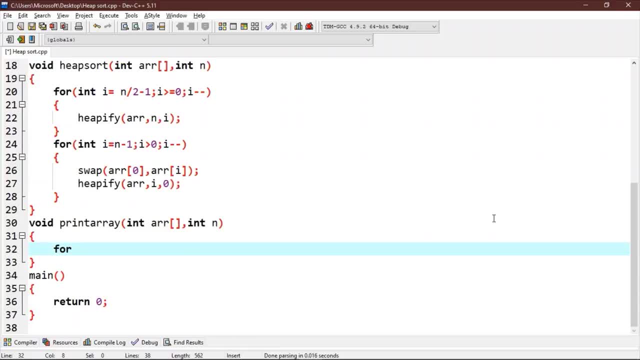 So for int i is equals to 0 at i-minus. So for int i is equals to 0 at i-minus. We will do cout arr, comma i dice, and a cout int l. Now let's write the code for the main block. 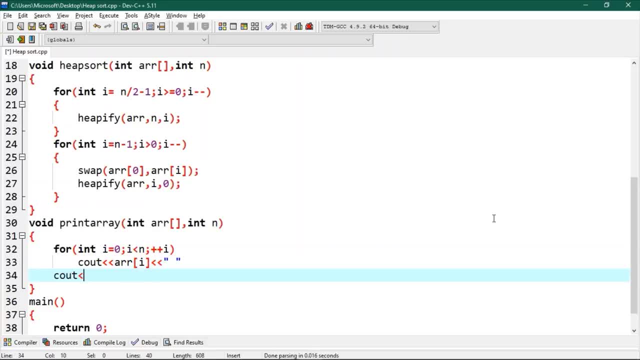 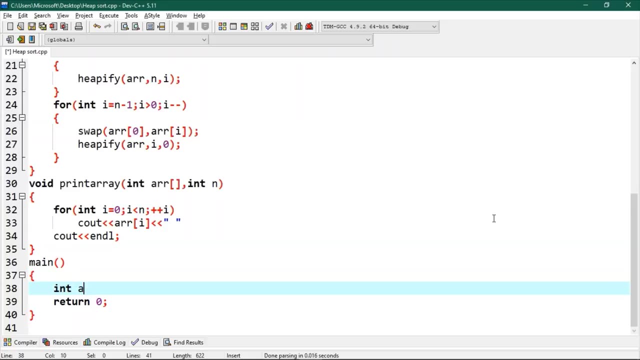 Now let's try drawing the main block. So int, comma i, comma e, we will vary the size Given this, save whisked. ARR is equals to. Now we will write a statement to find the size of this array. so int n is equals to. 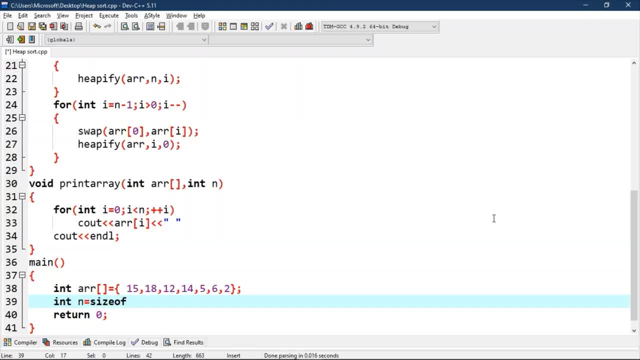 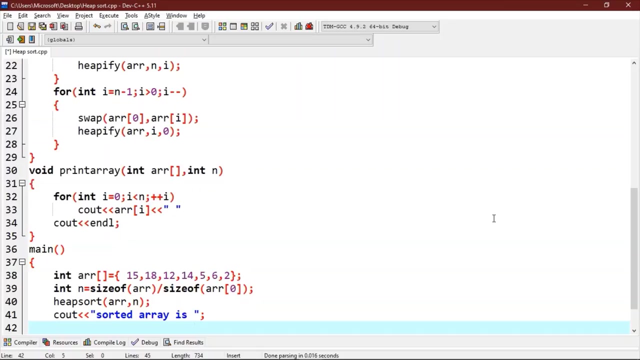 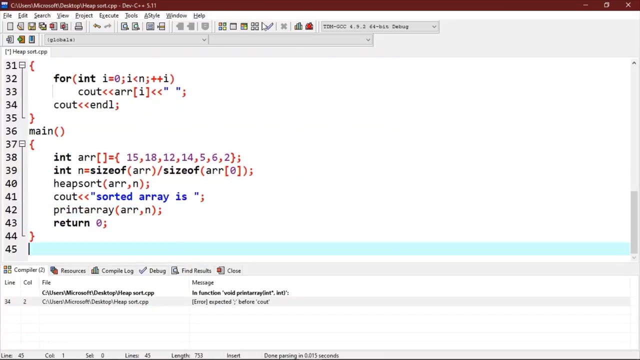 size of ARR divided by size of the first element of the array, ARR 0. Now we will call heap sort function, so heap sort for ARR comma n. Now let's print this array. so cout sorted array is print array at ARR comma n. Now let's try and execute this program. 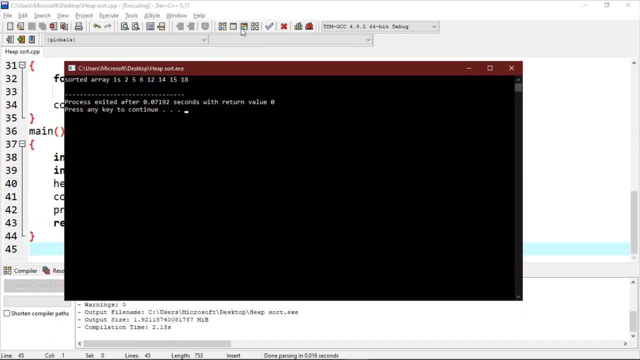 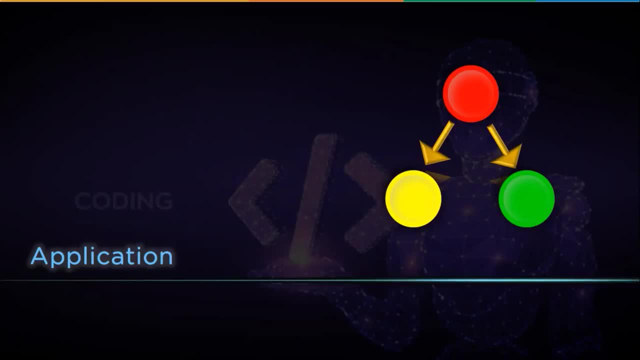 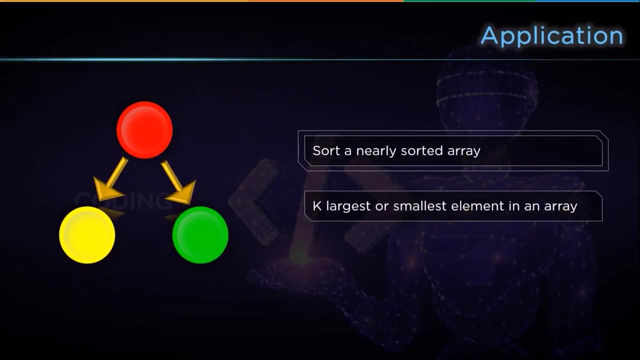 As you can see, our sorting function is working flawlessly. Now let's get back to our slides. Till now we have discussed the binary heap and the algorithm of heap sort. Now let's discuss some applications of heap sort. First up, It can be used to sort a nearly sorted series of data. 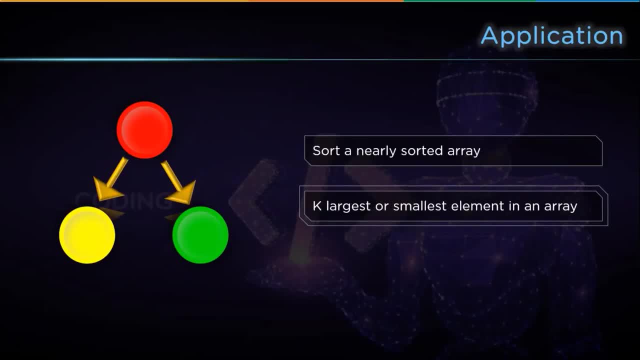 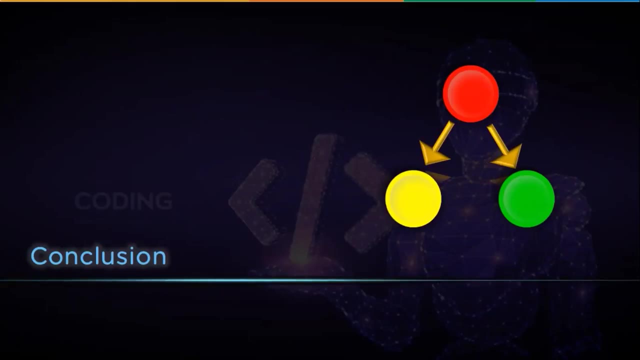 Next, It can be used to find minimum or maximum elements of the series with ease. Also, It can be used to solve problems which require some sort of priority At last. Let's sum up what we have learned from this session. First up, The tank. complexity of heap sort is